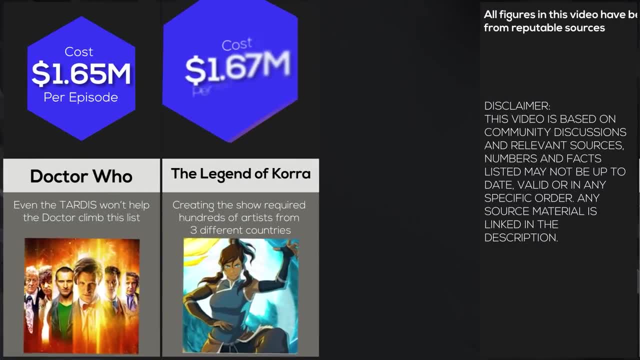 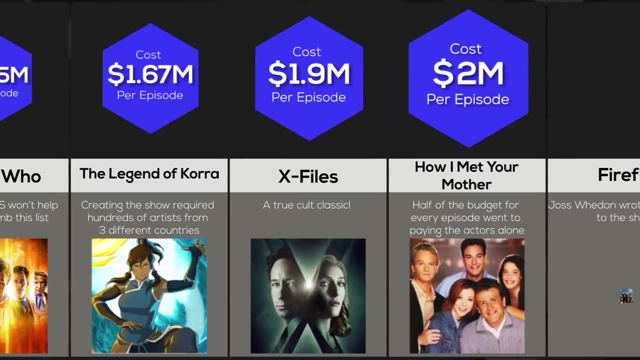 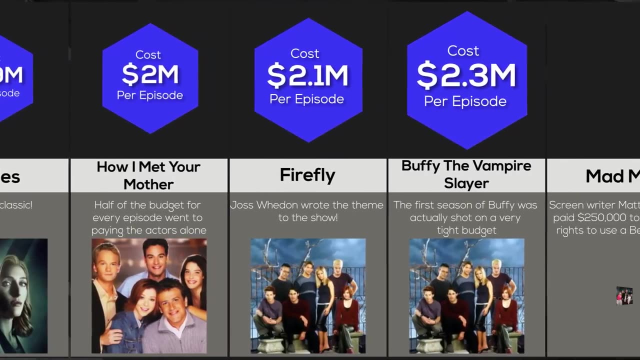 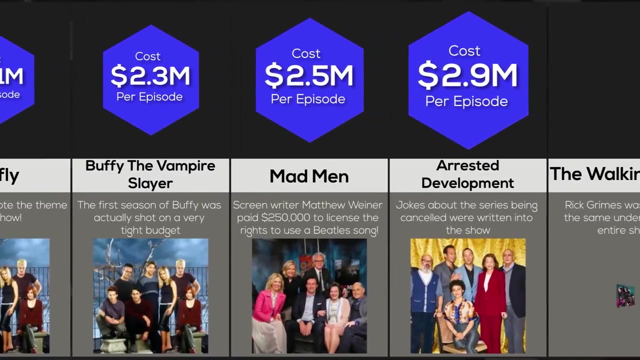 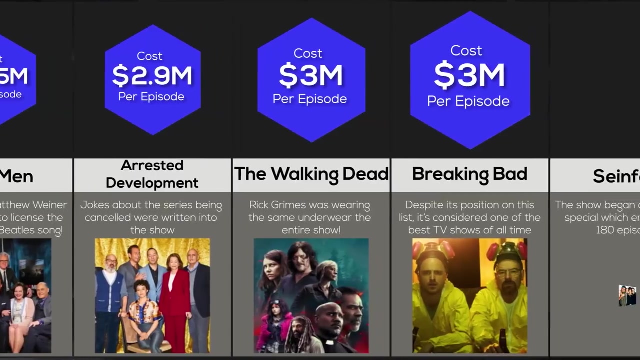 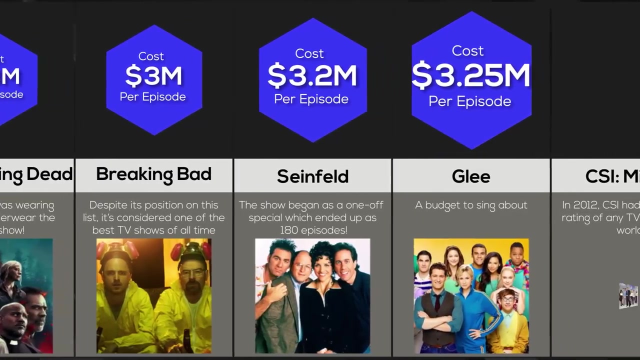 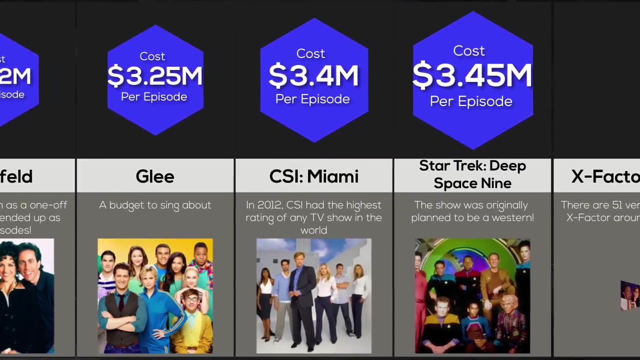 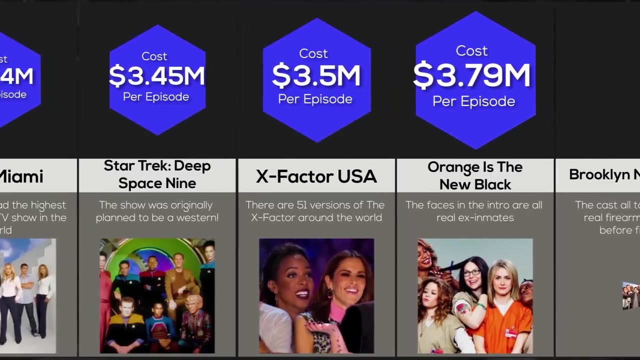 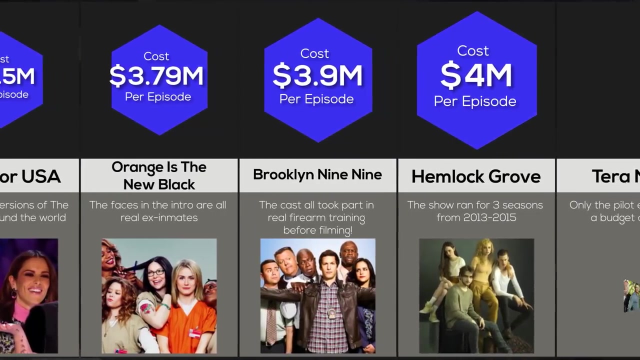 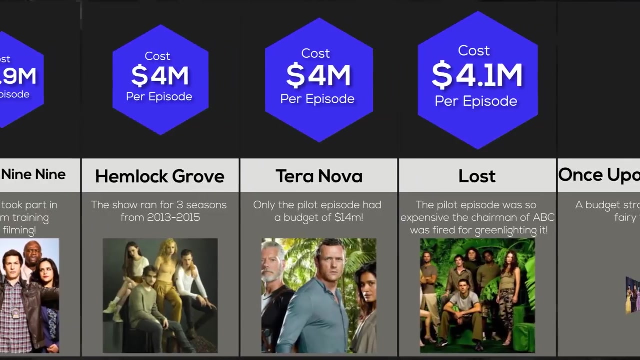 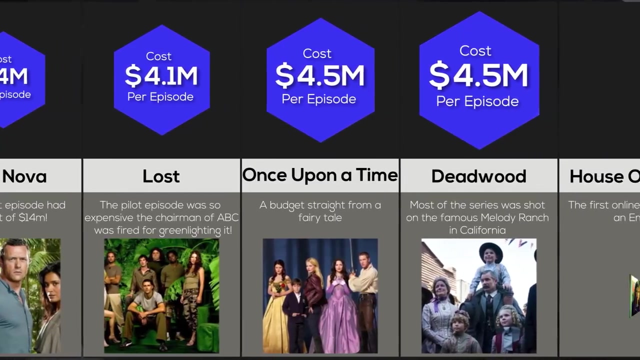 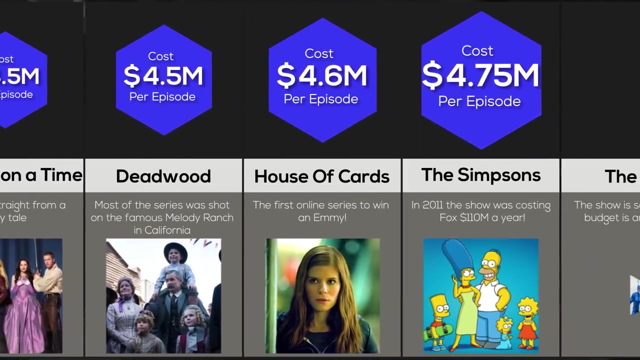 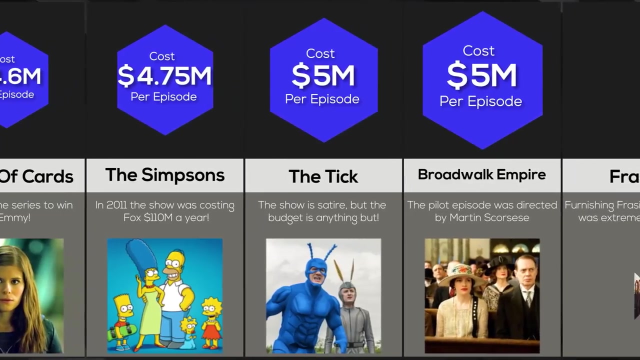 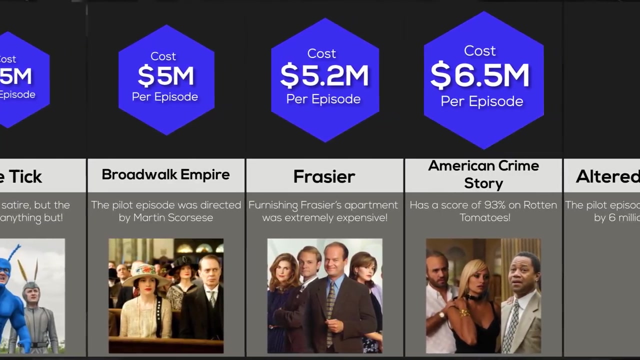 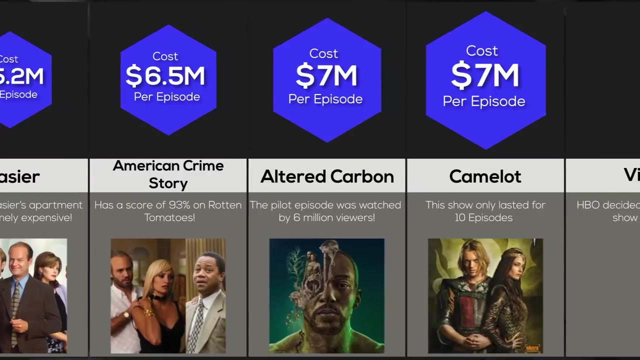 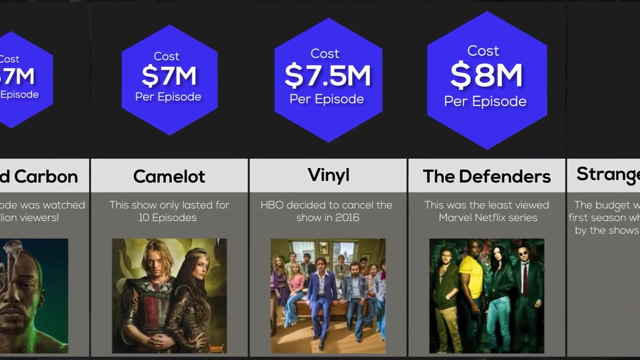 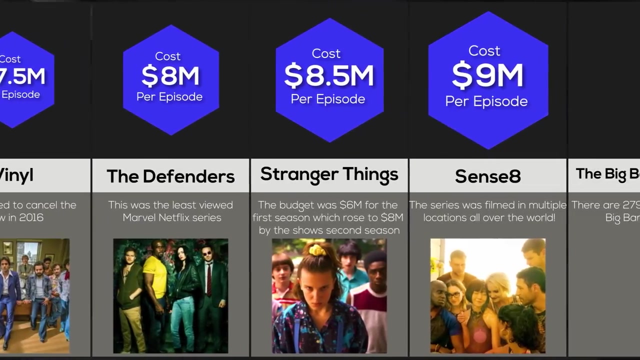 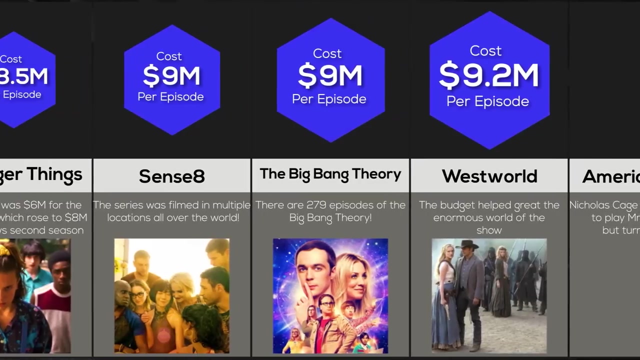 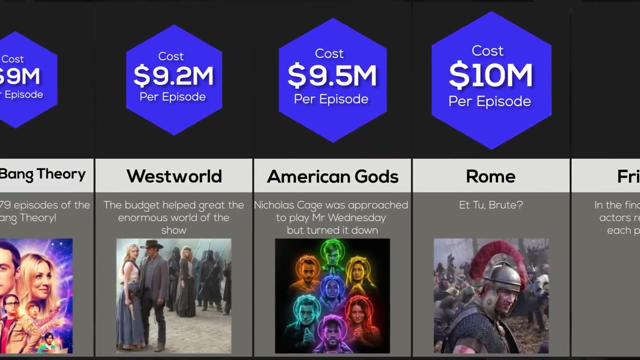 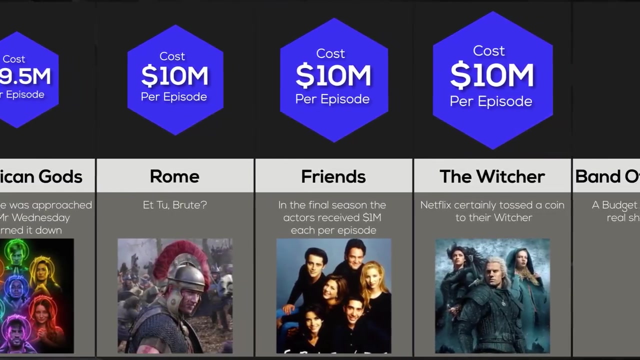 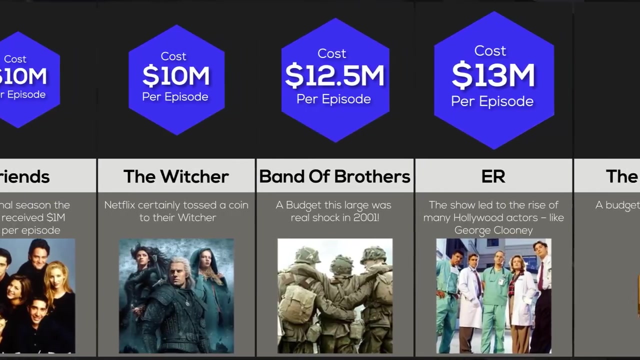 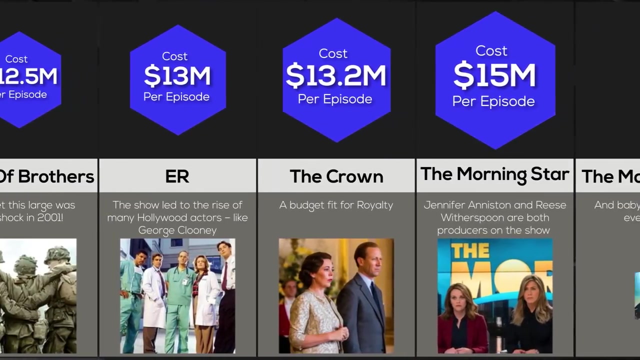 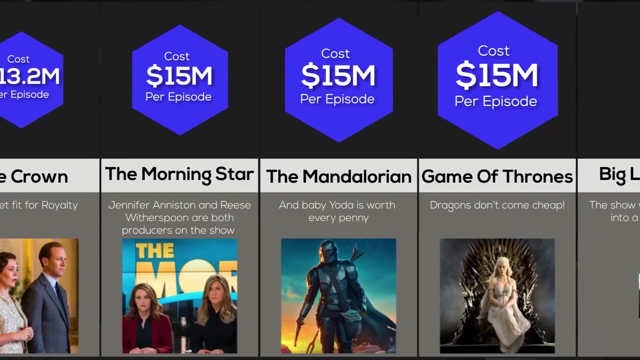 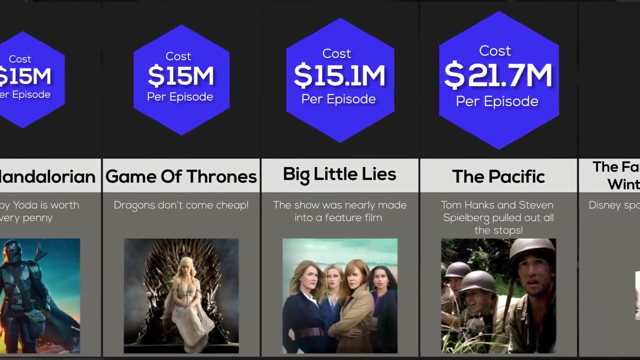 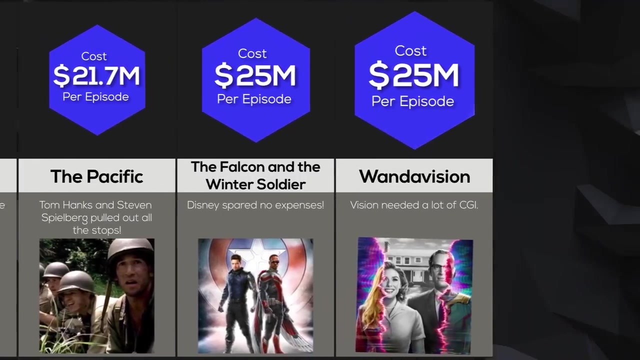 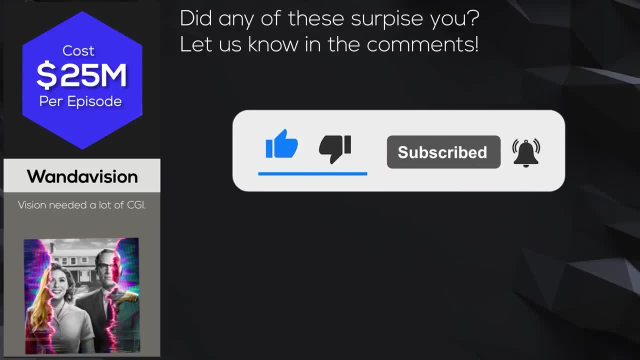 If you enjoyed it, then make sure to hit that like and subscribe button, Turn on those notifications and check out the next video. Check out some of our other stuff.